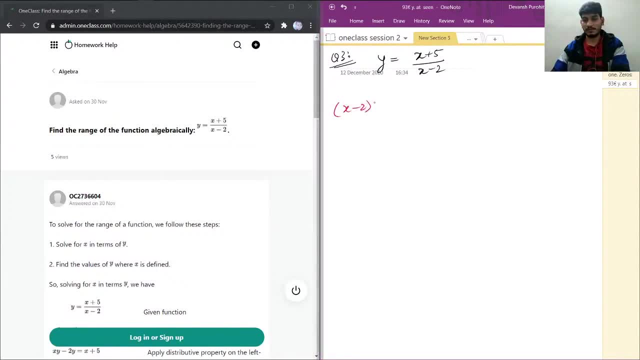 with x minus 2.. Y equals to x over x. Then this will become y x minus 2 y. So this will become y x. y will be x plus 5.. Now I will take x term on this side and I will take y term on this side. 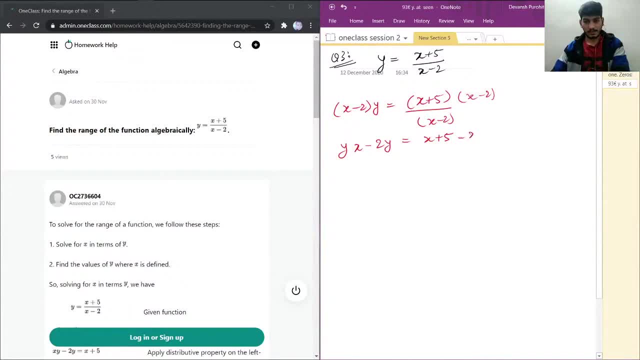 So basically I am going to take x term on this side and I will take y term on this side. So basically I will abstract x from both the sides and I will add 2 y to both the sides. So by this I will get x and x will get cancelled, Not x and x. So this will be y, x minus x. 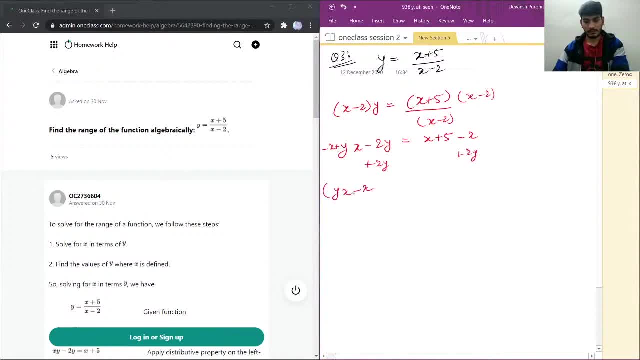 it and this will become um, we have x, x cancels, so 5 plus 2 y. i'm going to take y common. uh, i'm going to take x common here, and i will multiply both these sides with y minus 1, divide both the sides with, basically, y minus 1. 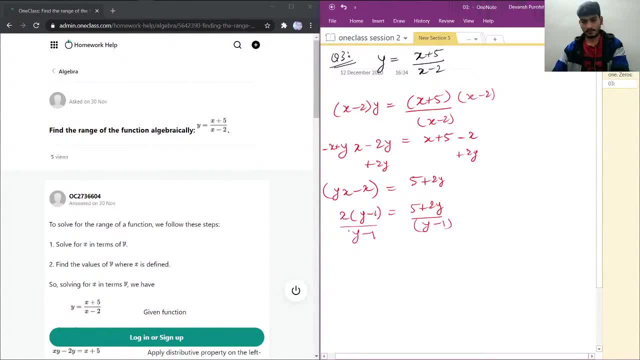 and here i get the equation. so, in this equation. so, finally, i have obtained the equation, uh, in terms of y, so that i can get the values of x. so in this equation, we can see here that x can be any number, but um, um, um. for this function to be continuous, uh, we should not have.